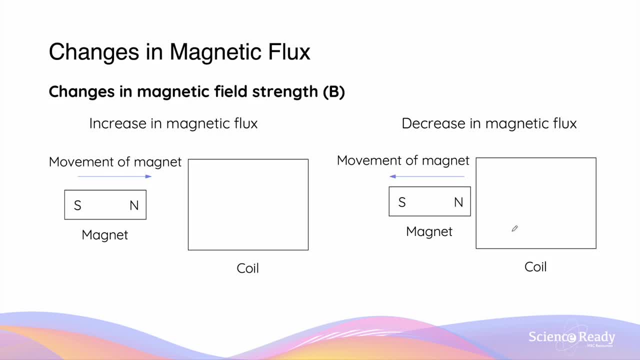 electromagnetic induction works. Let's go through some visual examples. If we have a rectangular coil and we move a bar magnet towards the coil, the coil will experience an increase in magnetic flux because the proximity of the bar magnet will determine the value of the flux density, that's 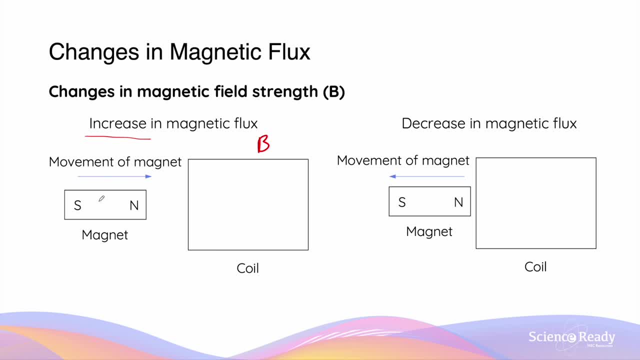 passing through the coil. The closer the bar magnet is, the higher the strength of the magnetic field. Vice versa: if the bar magnet is closer to the magnetic field, the higher the strength of the magnet is, and vice versa: If the bar magnet is moved away from the coil, the flux density or the 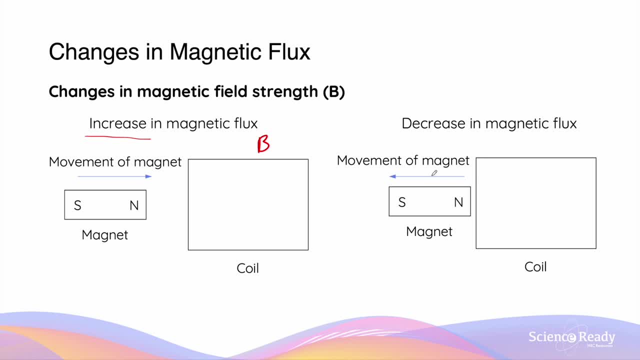 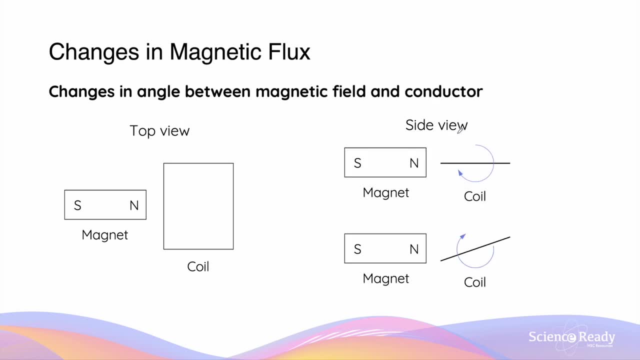 magnitude of the magnetic field experienced by the coil will also decrease and, as a result, it will experience a decrease in magnetic flux. In addition to the motion between the magnet and coil, the orientation or the angle between the coil and the magnet also matters. The bar magnet will of 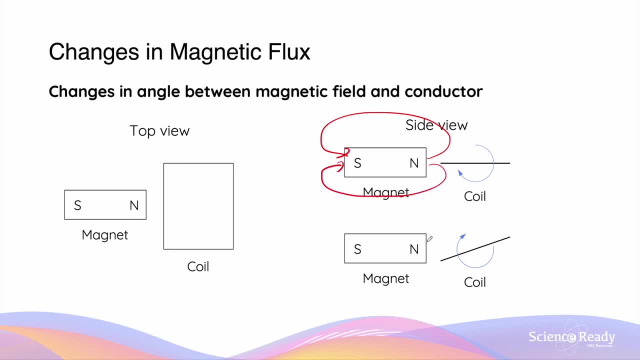 course generate its own magnetic field in the orientation from the north pole to the south pole. As shown. if we allow the magnetic field to move forward, the flow between the coil and the magnet will decrease pole. as shown: If we allow the coil to rotate, this is going to change the angle between its normal 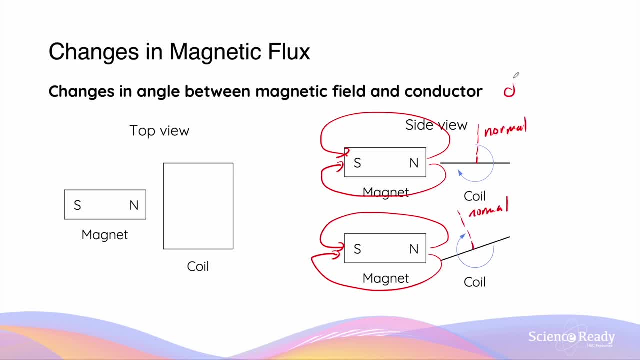 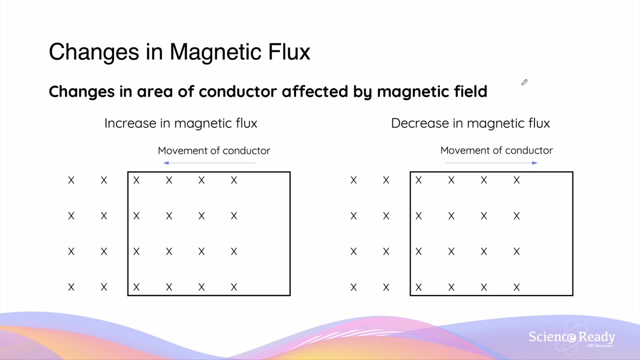 and the direction of the magnetic field. And since the value of flux is determined by this angle theta, as the angle theta changes, the value of the flux also changes. The third factor that determines the magnetic flux is the area. On the left hand side we have a rectangular conductor. 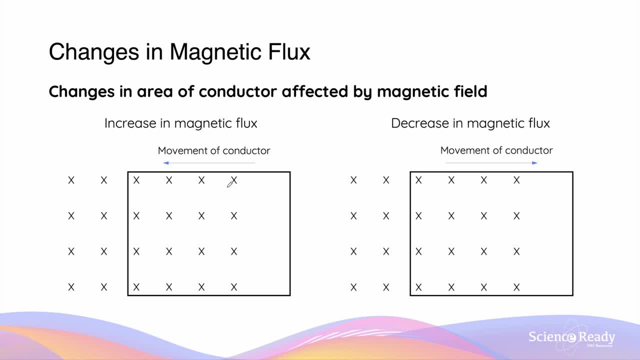 moving towards a uniform magnetic field, And as the conductor is moving towards into the field, the area of the conductor that's actually affected by the magnetic field is increasing. So as we have an increasing area, the amount of magnetic flux is also going to increase. 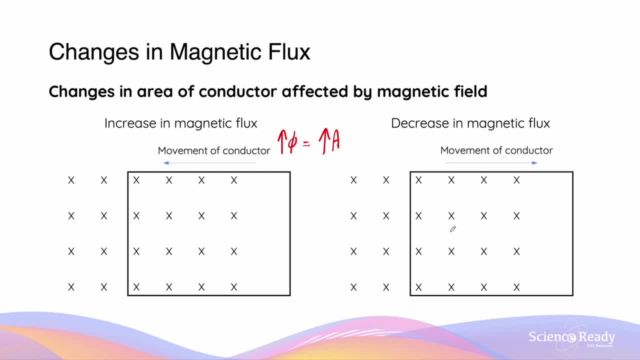 Vice versa. if we move the rectangular coil out of and away from the uniform magnetic field, the area of the conductor is also going to increase. So as we have an increasing area, the conductor that's being affected will effectively decrease And that's going to. 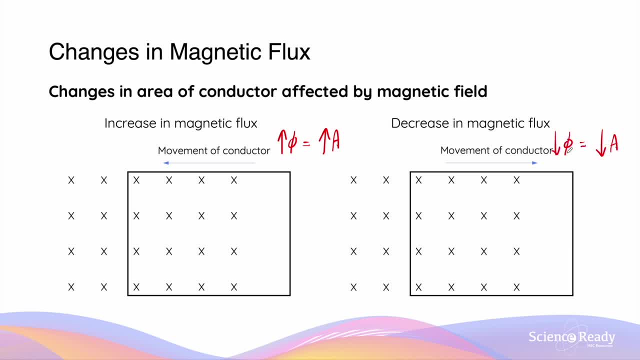 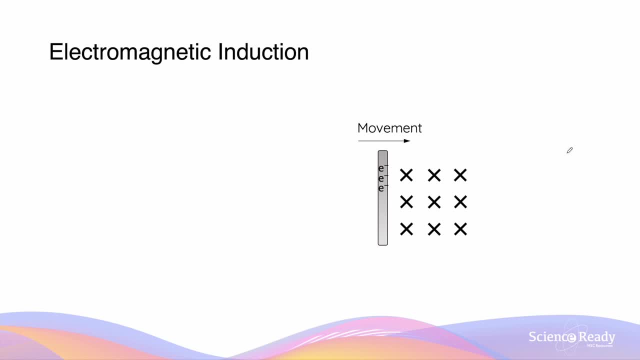 give us a reduced amount of flux passing through the conductor. So now that we've understood what magnetic flux is and how magnetic flux passing through a conductor can change, let's talk about electromagnetic induction. Suppose we have a rod containing electrons and we move this rod into a uniform magnetic field, as shown The charged particles. 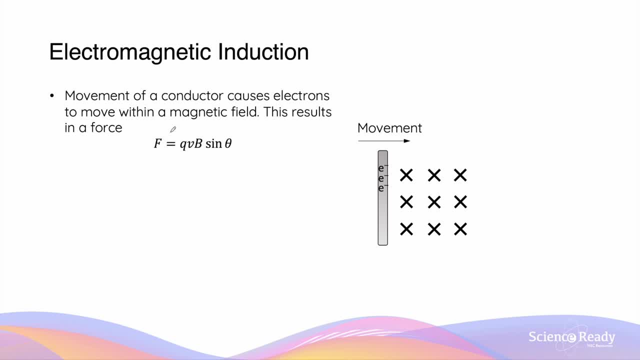 that is, the electrons that are in the conductor, are going to be affected by the magnetic field. The electrons in this conductor, as it's moving into the field, it will be acted upon by a force due to the magnetic field, And this force is given by QVB. sine theta, The direction of this force can 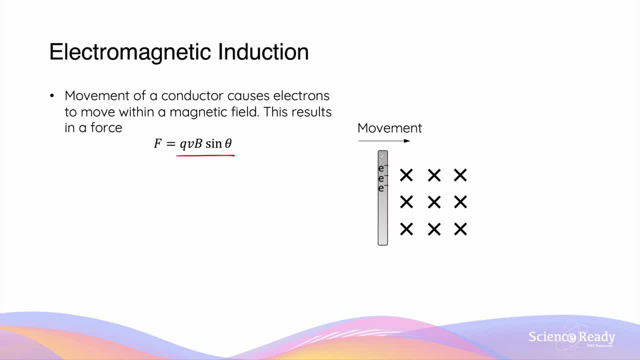 be determined using the right-hand palm rule. So if the electrons are moving to the right, we should point our thumb to the left-hand side of the screen. Our fingers will be in the same direction as the uniform magnetic field And, as a result, the force that's being produced due to the 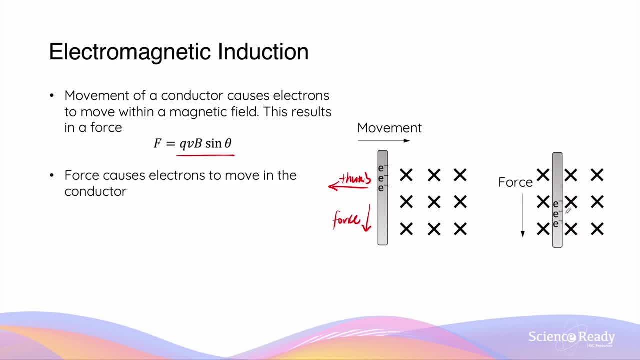 field will be going downwards And, as a result of this force, the electrons will start to move in the conductor. When we have these moving electrons, we will produce what we usually call an electric current. The direction of this induced conventional current is typically defined in the. 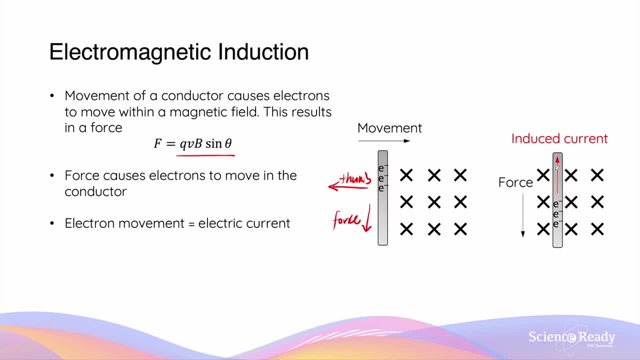 opposite direction as the movement of the electrons. So although the electrons are moving downward due to this force, the current actually moves upwards. This phenomenon, where a conventional current is produced due to the forces acting on the electrons in the conductor, is an example of. 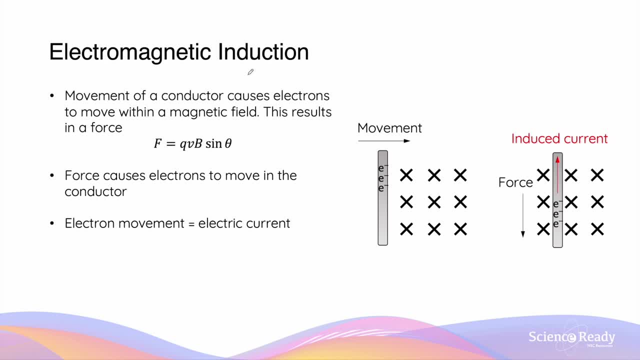 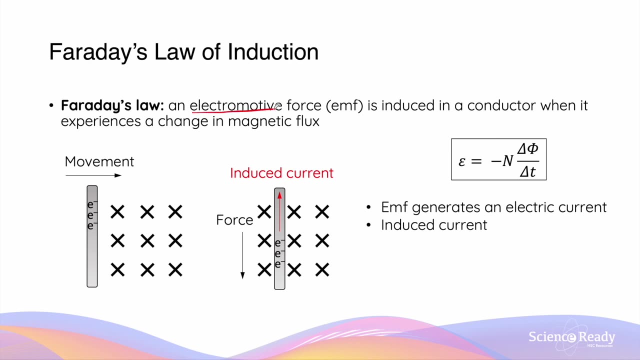 what we call electromagnetic induction. The word induction refers to the fact that we have produced current by simply moving a conductor within a magnetic field. Faraday's law of induction states that an electromotive force- EMF for short- is induced in a conductor when the conductor is. 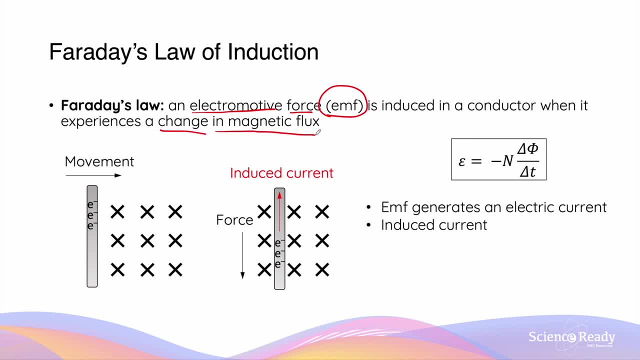 experiencing a change in magnetic flux. In the previous example, when the rod containing electrons is moved towards the uniform magnetic field, it will experience an increase in flux because a greater area of the conductor will be within the field, According to Faraday, when this 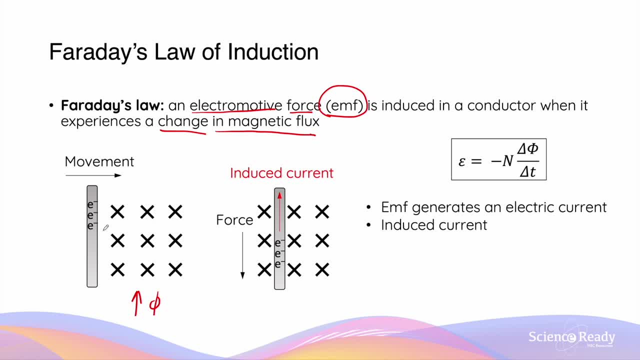 conductor experiences any type of change in flux, including an increase in flux, there will be an EMF, which is also very important for the conductor to experience an increase in flux. The EMF is the voltage that's being induced within the conductor, and this voltage, or EMF, 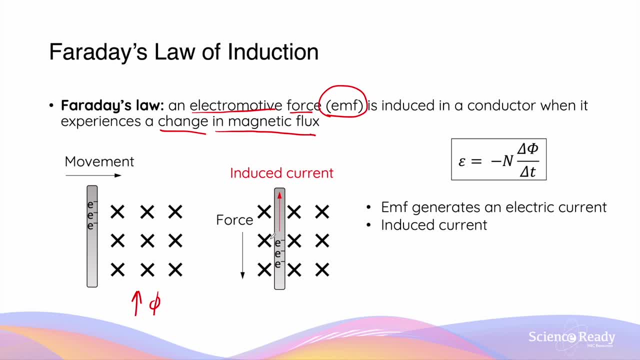 will cause a current to be produced. Mathematically, Faraday's law is expressed as the following equation: Epsilon stands for. the EMF is equal to minus n being the number of turns of the conductor times by the change in flux over the change in time. This equation tells us that the magnitude 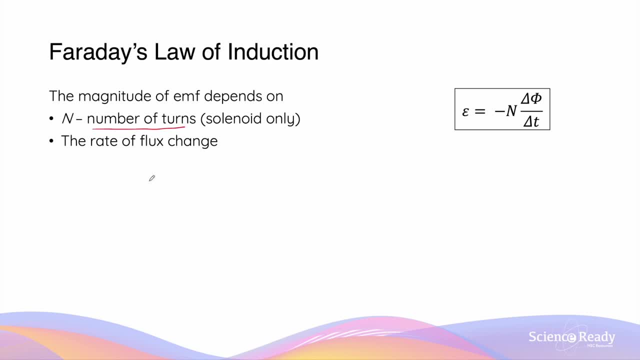 of EMF depends on the number of turns of the coil, which is typically only applicable when we look at solenoids rather than straight conductors, and, more importantly, it also depends on the rate of flux change. So that's, how quickly is the amount of magnetic flux changing? 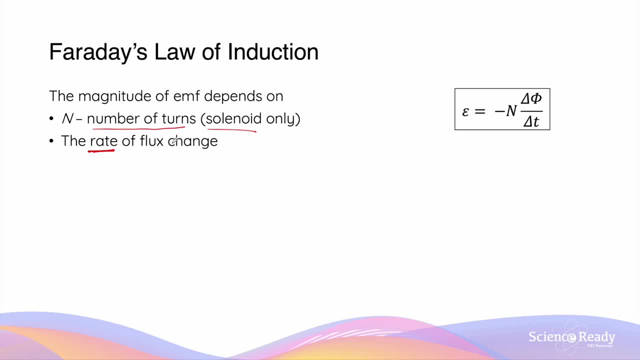 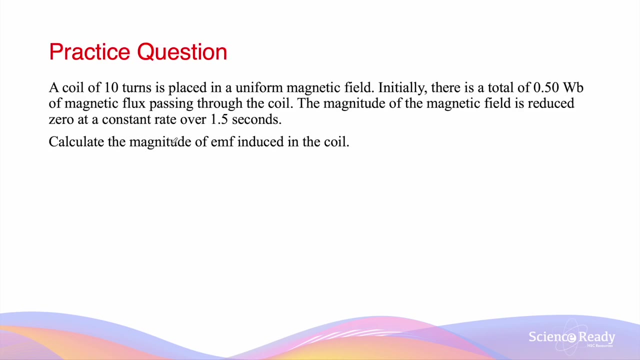 The faster the flux is changing, the greater the magnitude the EMF will be and consequently, if you have a greater EMF, you will likely have a greater EMF. Let's have a look at how we can use Faraday's law's equation in an examination question. 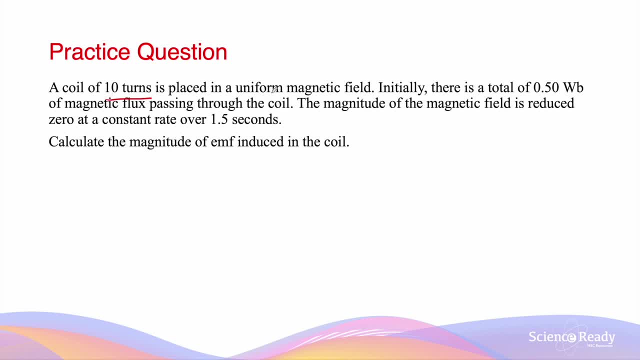 So we have a coil of 10 turns placed inside a uniform magnetic field. Initially, there's a total of 0.5 webers of flux passing through the coil. so this is my initial amount of phi. The magnitude of the field is reduced to 0 at a constant rate over 1.5 seconds. so this is my final amount of flux, which is 0.. And the time is 0.5 seconds. So this is my final amount of flux, which is 0.. And the time is 0.5 seconds. So this is my final amount of flux, which is 0.. And the time. 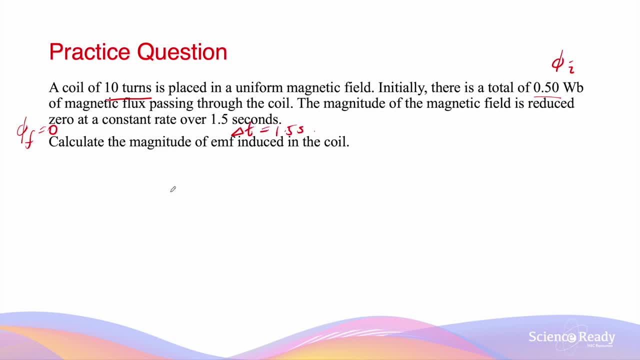 that's taken to do so is 1.5 seconds. So Faraday's law is equal to minus n times by delta phi over delta t or the changing time, So minus 10 turns multiplied by the changing phi. So the changing flux is the final minus the initial divided by the changing time. 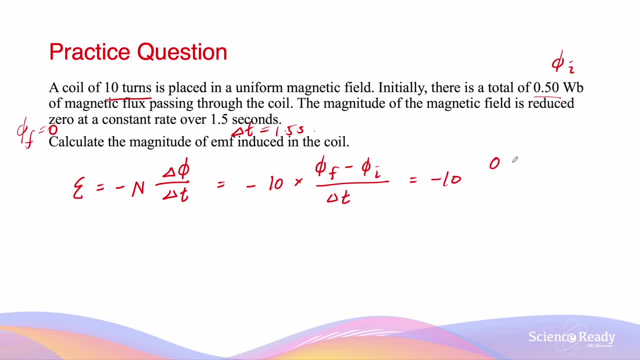 So this is equal to 0 minus 0.5 webers divided by 1.5 seconds, And this gives me a 3.33 volts of emf. This emf, if it's induced in a coil, that's already in a. 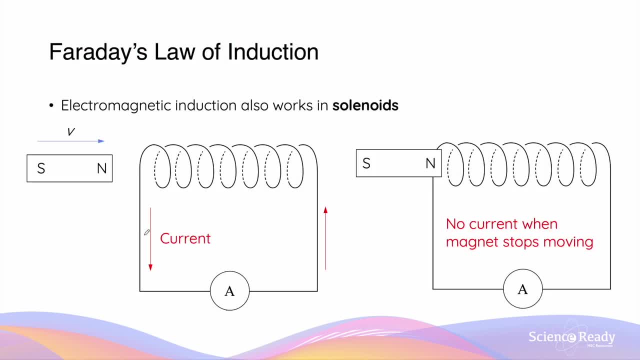 closed circuit will produce a current. Besides straight conductors, Faraday's law of induction can also be demonstrated using solenoids or coils. This is usually demonstrated by using a bar magnet and a solenoid connected to an ammeter which can detect current When the bar magnet is.